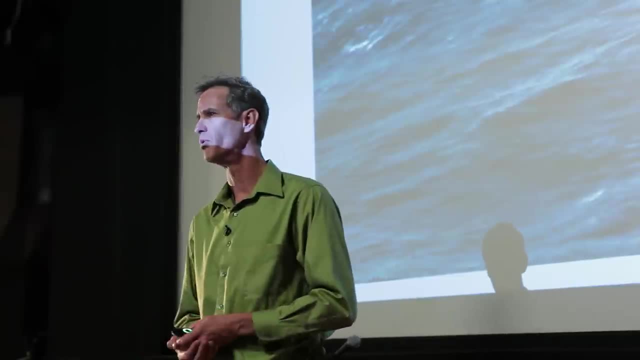 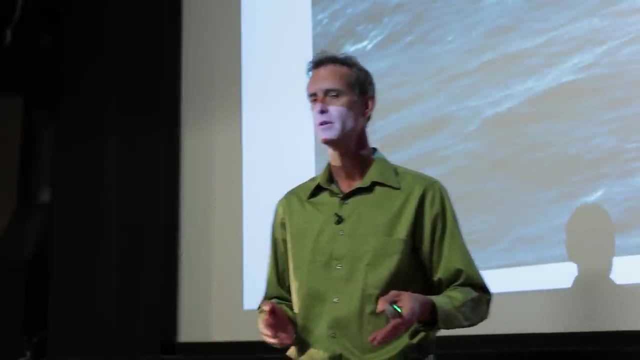 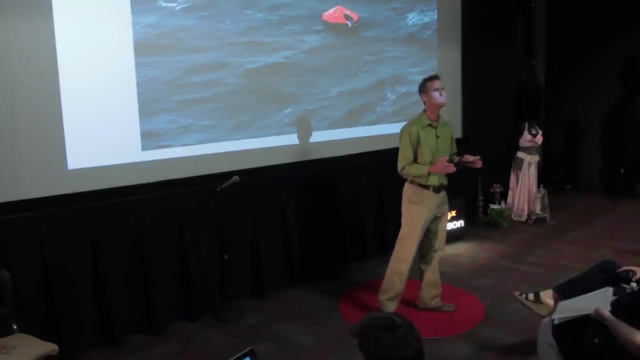 a few containers of food and some bottles of water on board, And periodically they pick up more survivors. So what's going on here? Well, the demand for food is increasing as the survivors accumulate, But at the same time the supply is diminishing from consumption. So what should be done here? 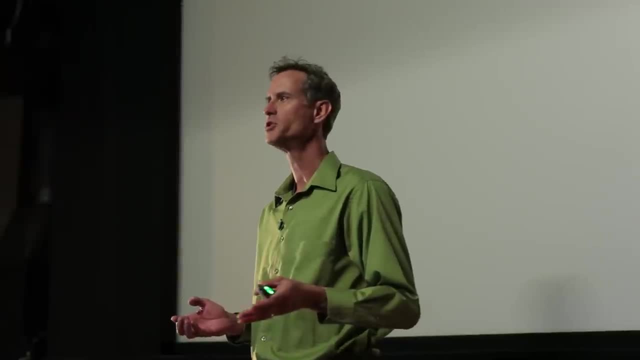 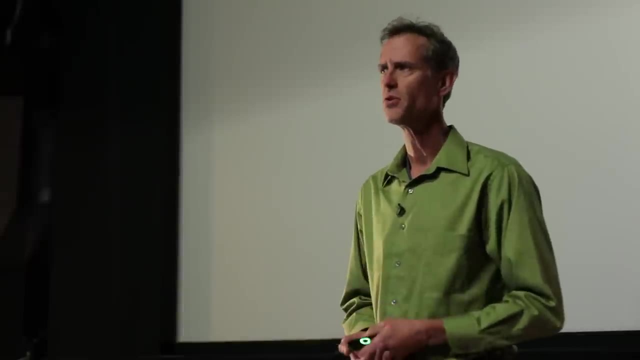 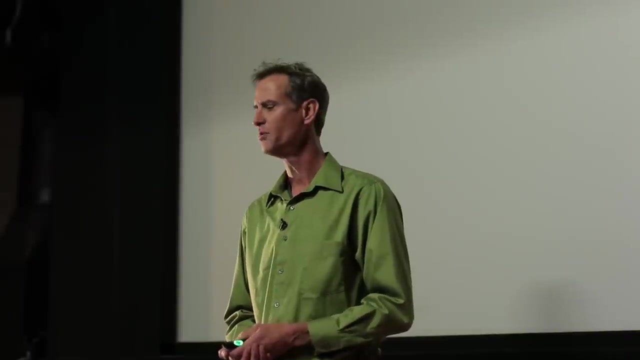 Should everyone on board get the same amount of food, Or should the injured or the sick or the elderly get more than the others? So these are difficult questions. So I work at the University of Arizona and I teach a class for the Honors College called Human Reproduction and the 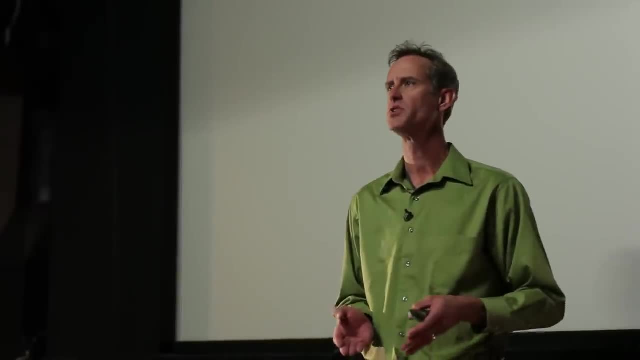 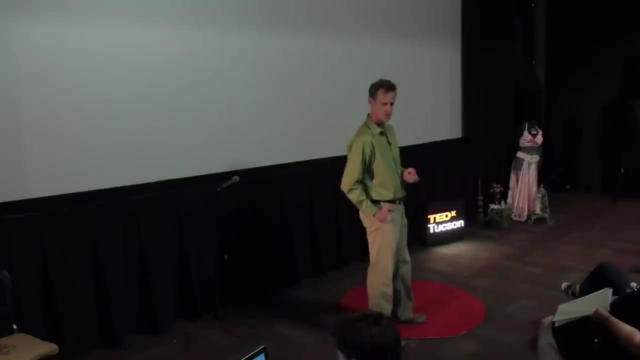 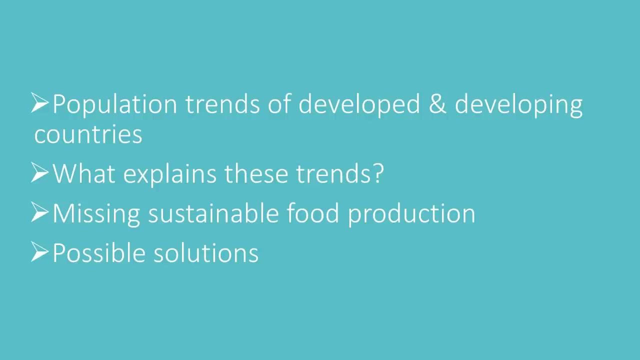 Environment, And I'd like to share with you some perspectives that I've gained from teaching this class. So the topics for this talk will be the following: I'll be talking to you about trends of population versus developing countries, the characteristics that help define those trends, 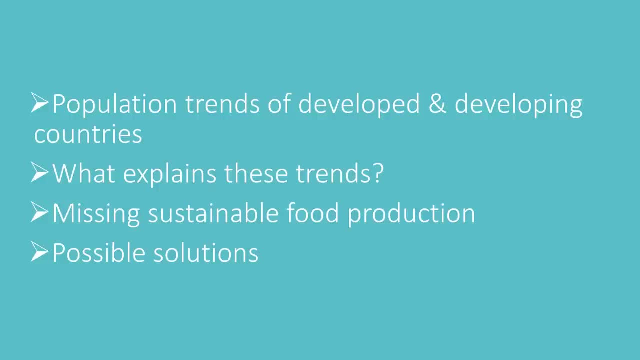 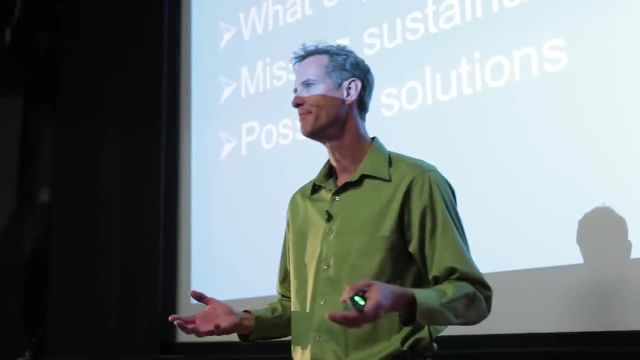 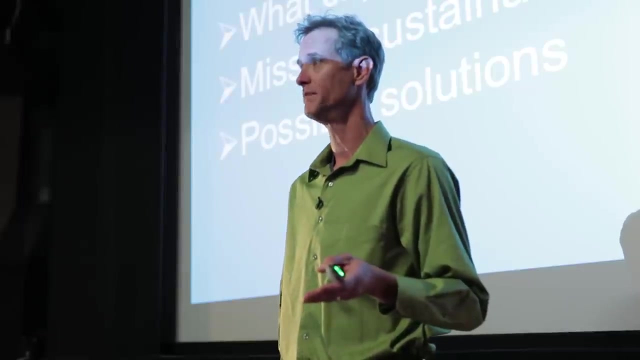 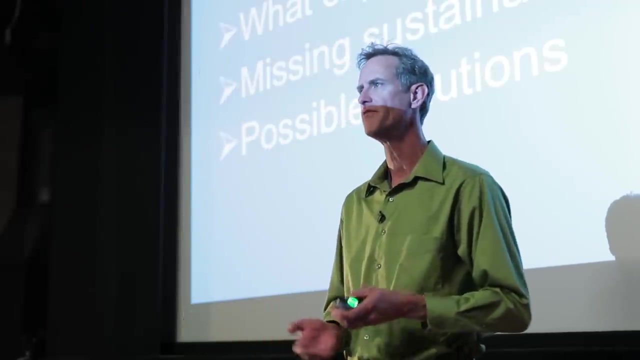 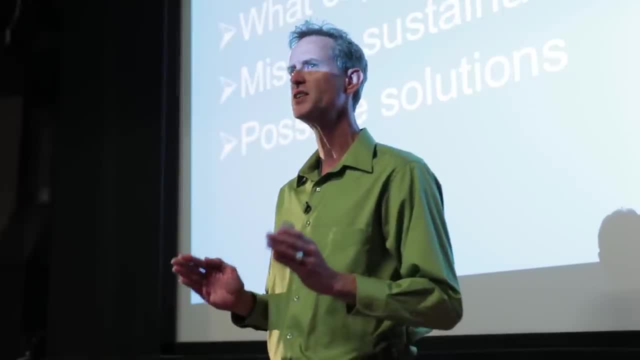 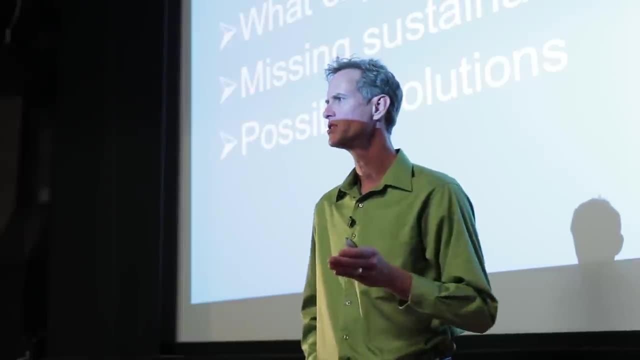 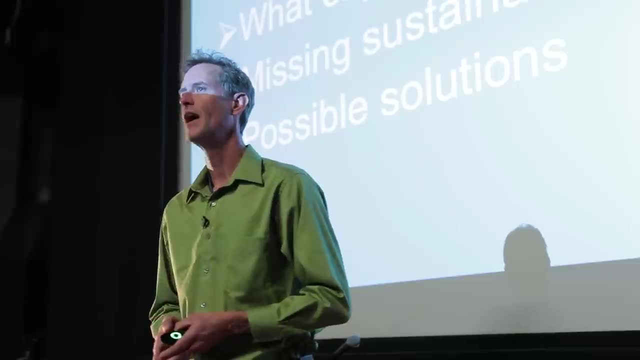 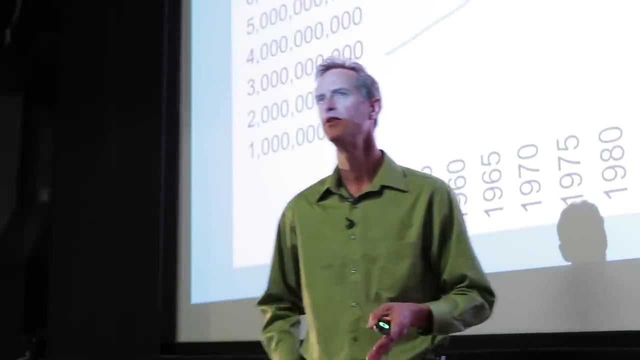 what I've said in the context of your own life and start a conversation with others about it. Now, we'd all agree there are more people now than ever before in the history of our planet, And as the population grows, so does the population of the region. So that's one of the main things I would like toKIING to address to you today. I'd like to mammolize just exactly where we are right now, To Bernie Sanders or to Michael Van Itter or to the television 101.. 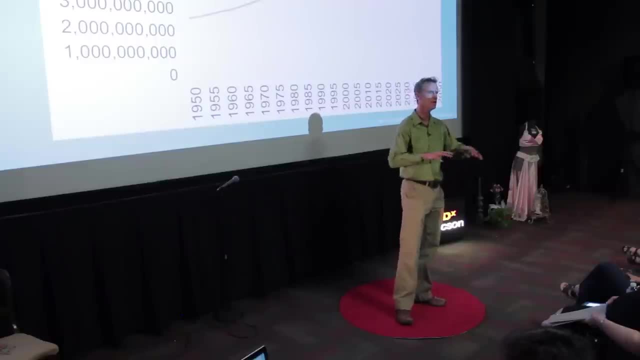 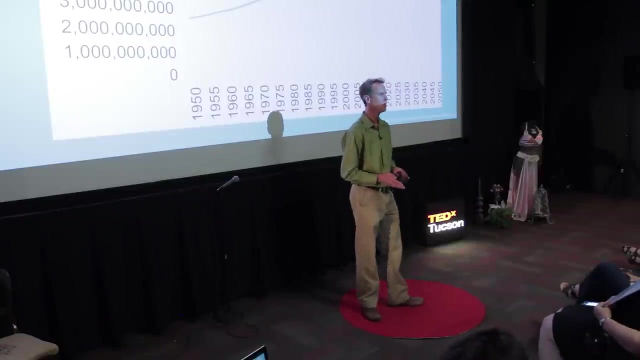 Thank you very muchальной the demand for food, But are we all evenly distributed around the planet? Well, no. In developed countries, in fact, the average family size is decreasing, But these are the families with the easiest and the most access to food. In developing countries it's a different. 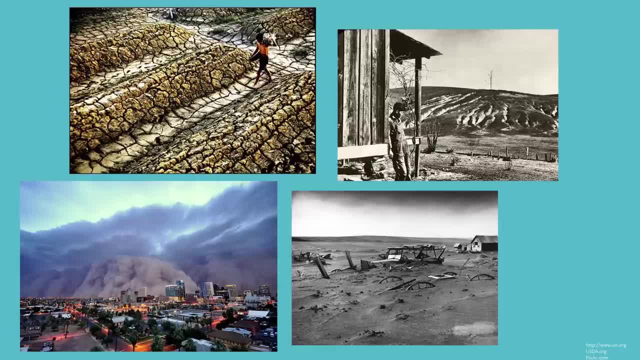 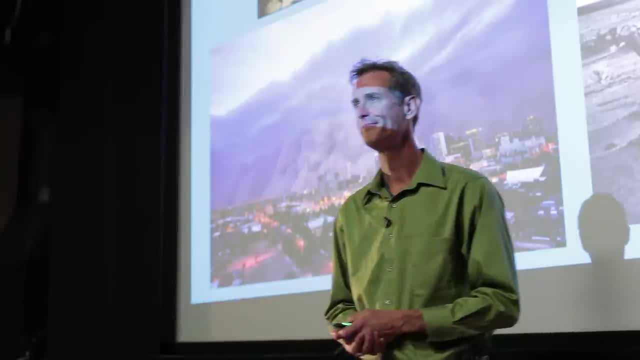 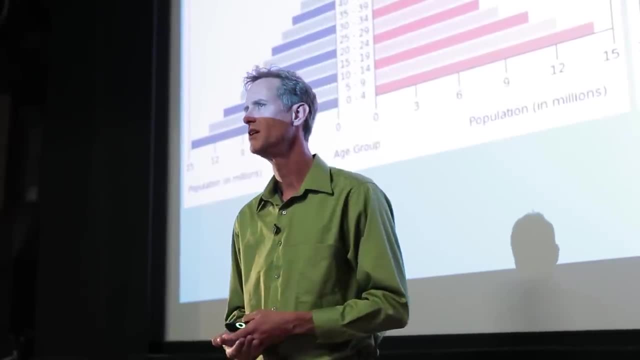 story. The average family size is much bigger and land degradation has had a significant input on food production. I'd like to share with you some stats that I put together, So this is based on 2013 census data. These are age population pyramids, So they show the 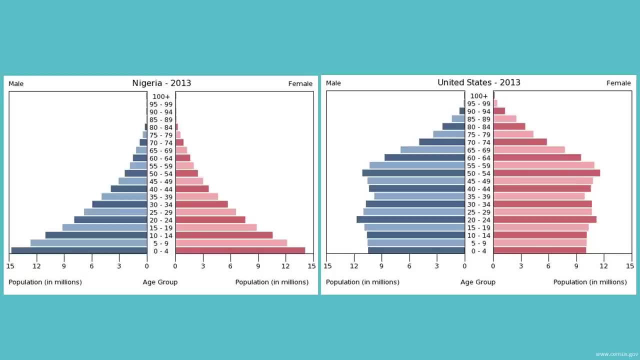 age population distribution for individual countries, And on the left you see Nigeria, a developing country, and on the right you see that of the United States. And in the next slide you see a similar comparison between Afghanistan and Germany- Slide 4.. 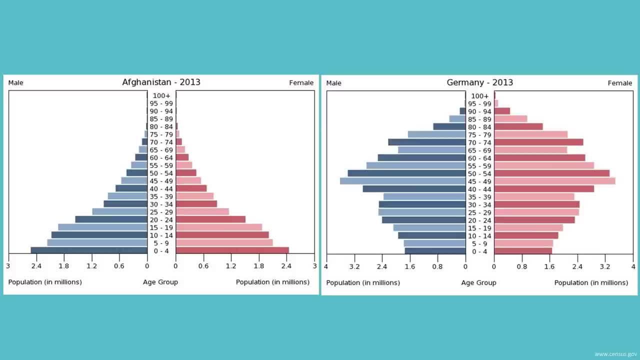 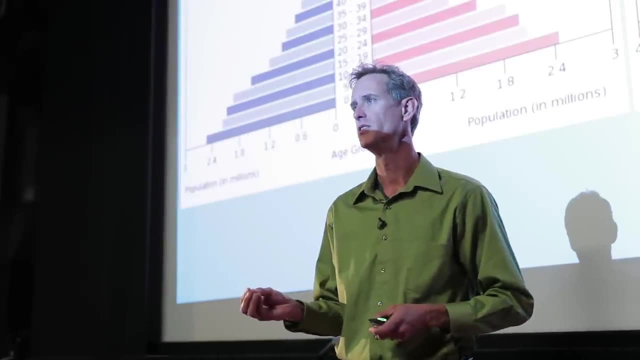 Now notice how in the developed countries the population age distribution is fairly uniform, with the pronounced bulge of the baby boomer generation. But notice how in the developing countries the majority of the population is in the younger age classes And in. 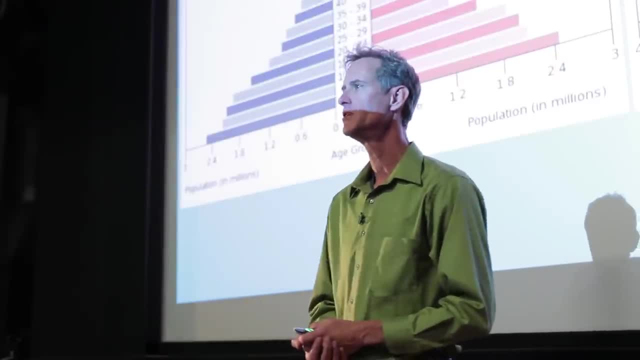 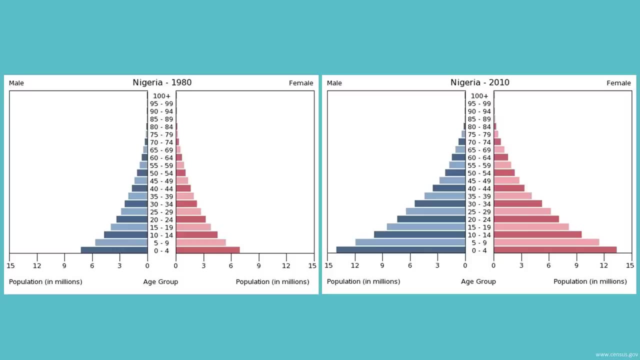 fact, in Nigeria, Africa's most populous country, over half of the population is under the age of 15.. Slide 5.. Now this trend has been occurring for decades, as shown here by Nigeria from 1980 to 2010.. 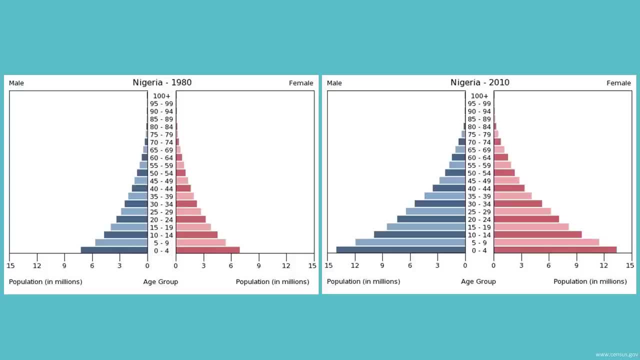 Except now it's even more pronounced. Now, childhood mortality, perceived or otherwise, goes a long way to explain this, And the lack of health care means that parents want more children to care for them when they're elderly. Now, it's not that families are having more. 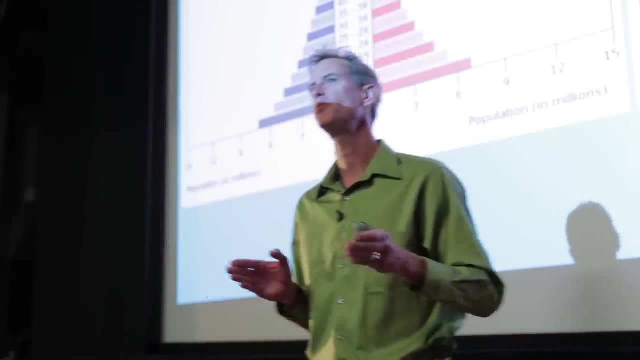 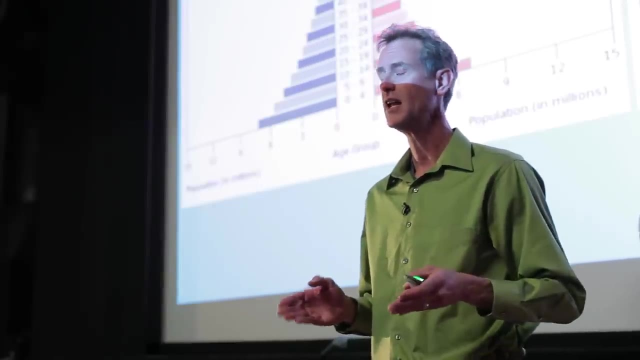 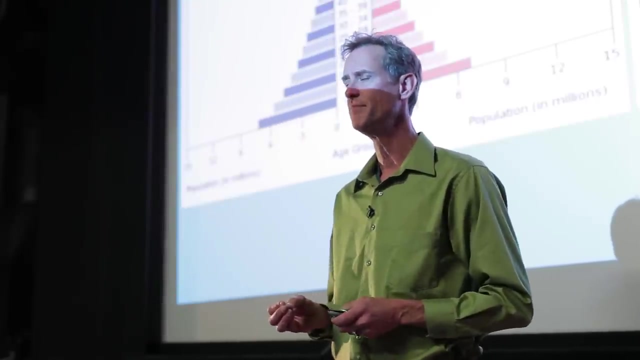 children. now Slide 6. It's that they're having the same number of children as their parents and their grandparents did, Except now there's more of them having those children. And how many children? Well, the average number of children right now in Nigeria is six, But often as many as ten. 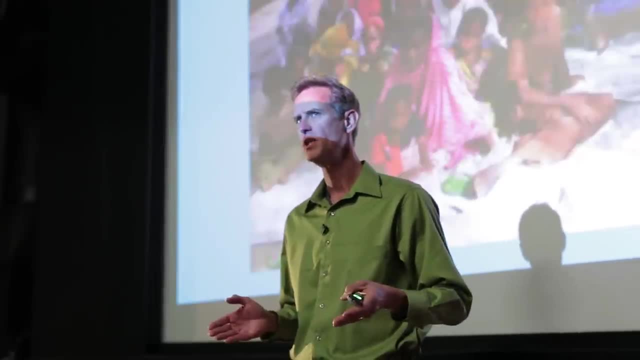 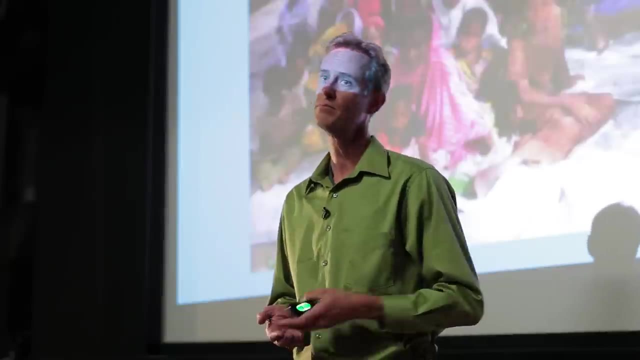 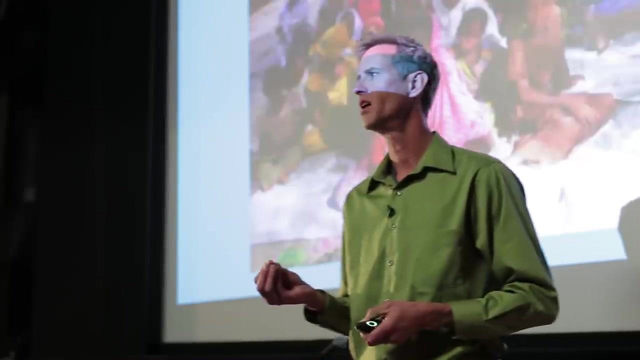 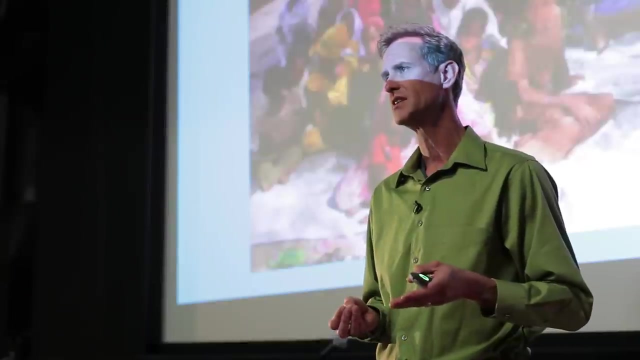 Slide 7.. So that leads me to ask: why is it in developed countries that the average family size is smaller? Well, prosperous economy, a developed infrastructure and relatively low income. Slide 8.. And so, despite the tax credits given in the United States per number of children, the average family size has decreased as the people in this country recognize the direct connection between a standard of living and the number of children And to maintain that standard of living, the average family size is maintained so that both parents work And that's harder to do with the larger family. Slide 9.. 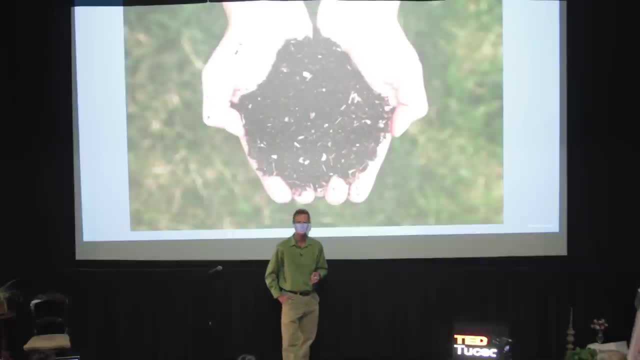 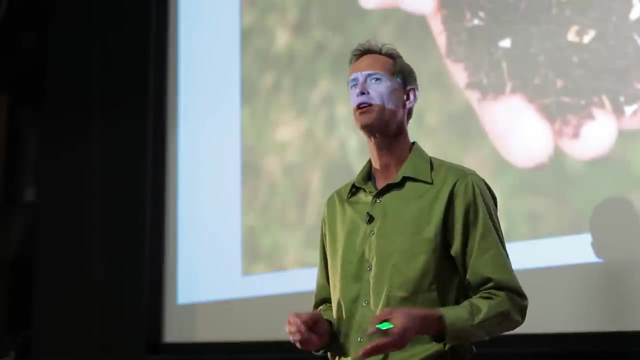 So that leads me to supply my next topic. According to the United Nations Food and Agriculture Organization, 99.7% of the food that we eat is derived from soil. Yet land degradation directly related to food production has been occurring worldwide and costs billions of. dollars And in the United States alone, the average annual cost- well, it's not average but it ranges- but the annual cost is between 9 and 44 billion dollars in lost revenue, damages and efforts to reverse that erosion. 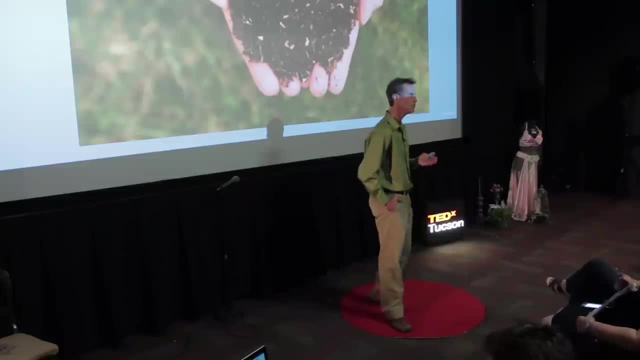 Slide 10.. Now let's face it: food production is destructive to the environment. Natural vegetation is removed, the surface of the land is re-contoured and the very structure of the soil is destroyed from tillage to promote planting. Slide 11.. And soil fertility. Wind and water erosion take their toll as well, And each year an area of land that could be used to grow plants for food is lost to soil erosion, And that amounts to an area the size of the state of Iowa each year. 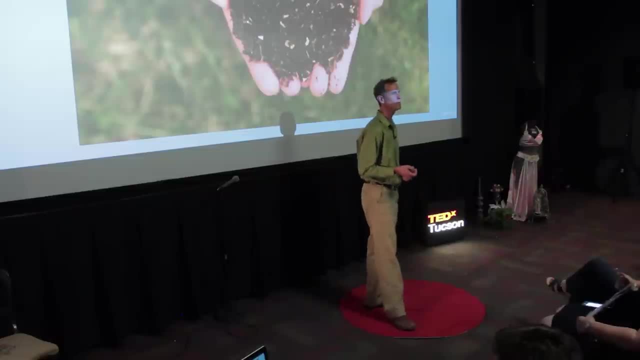 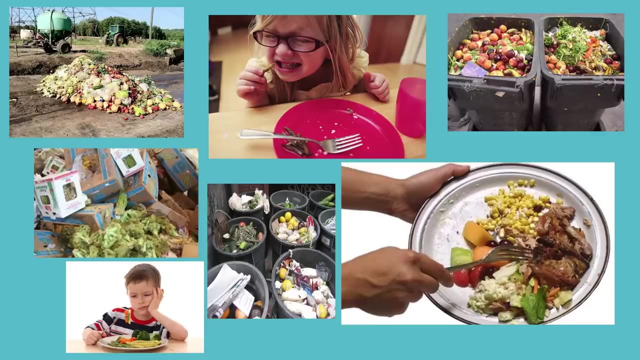 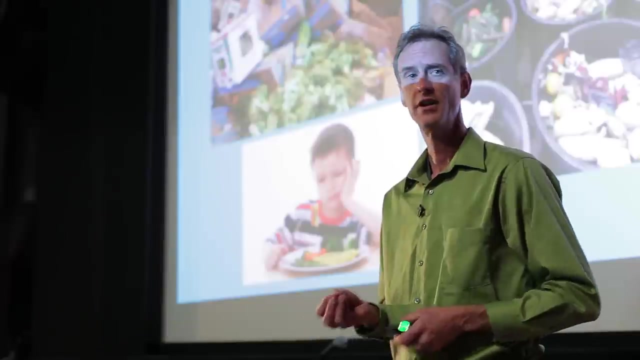 Slide 12.. So, even if that food is produced, where does it end up? Well, let me ask you this: your last trip to the grocery store, how much food did you buy, And what decisions led you to purchase that food? And then, finally, how much of that food? 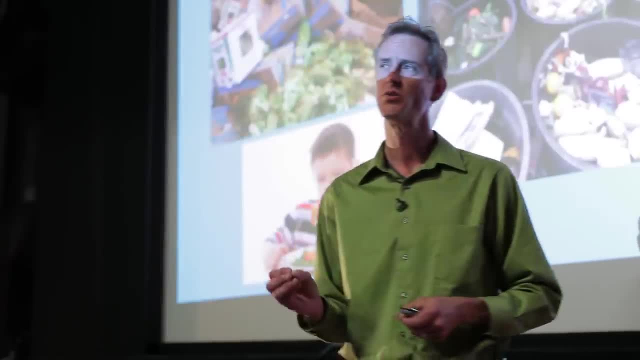 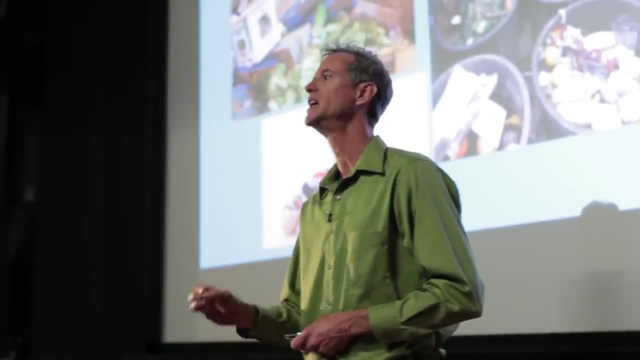 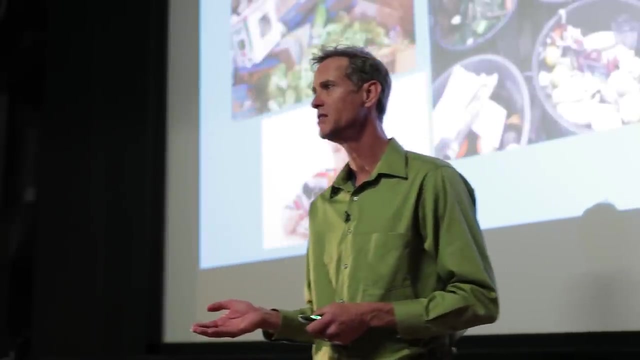 that you purchased went uneaten. Now, according to a recent USDA study in 2010,, 31 percent of the food produced in the United States went uneaten. It was lost due to rot or contamination at the source. retailers rejected it due to blemishes or an unsuitable color, and the 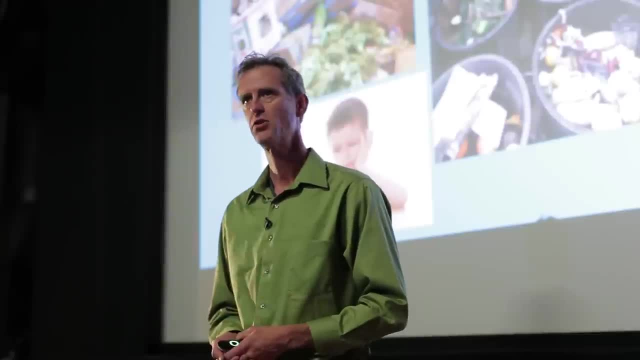 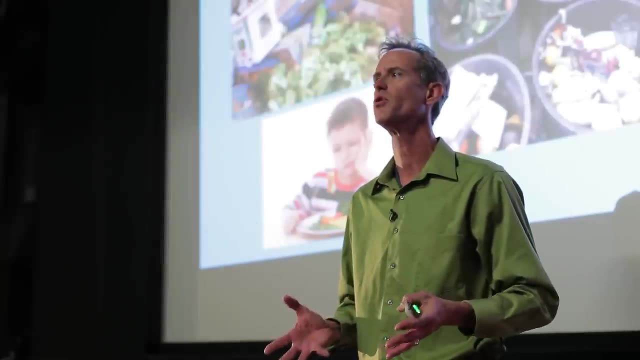 rest was purchased by consumers but went uneaten. Slide 13.. Slide 14.. Slide 15.. Slide 16.. Slide 17.. Slide 18.. And according to the UN Food and Agriculture Organization, this trend continues all over the world, with a third of the food produced going uneaten. 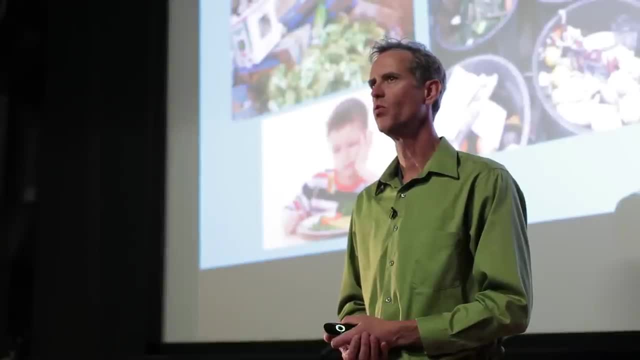 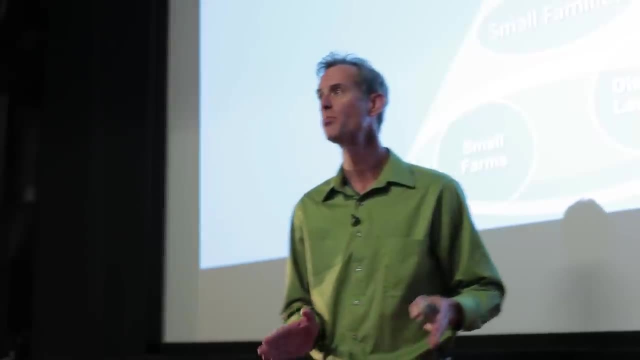 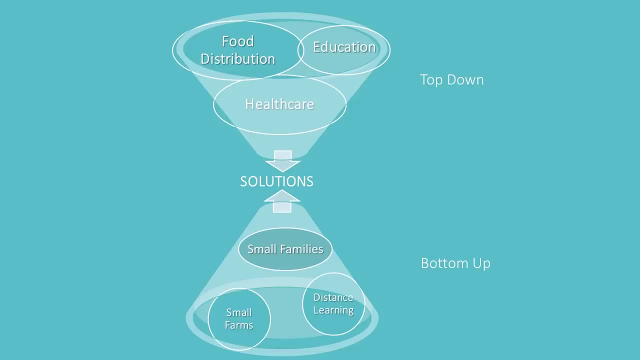 Slide 19.. Slide 30.. So what can be done to reduce the demand for this food? Well, broadly speaking, two approaches are possible. The top-down approach has governments and or religions determining how many children should be born in each household, either explicitly by law, as, in my opinion, the right way. 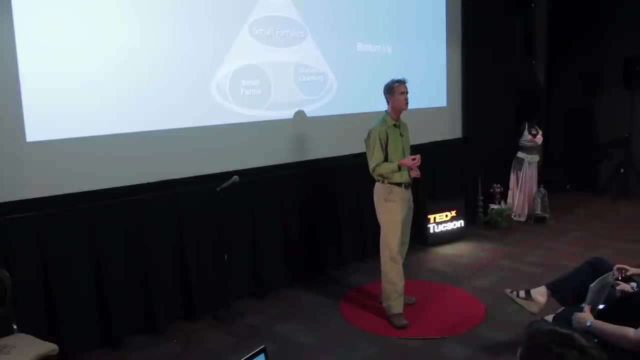 as in the case of China, for example, or implicitly, by control of access to resources such as food, certainly, but also education and health care. birth control measures And other incentives include tax breaks, subsidies for sterilization or a campaign by the media. 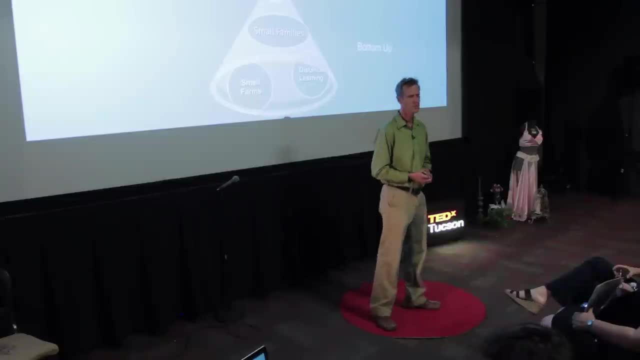 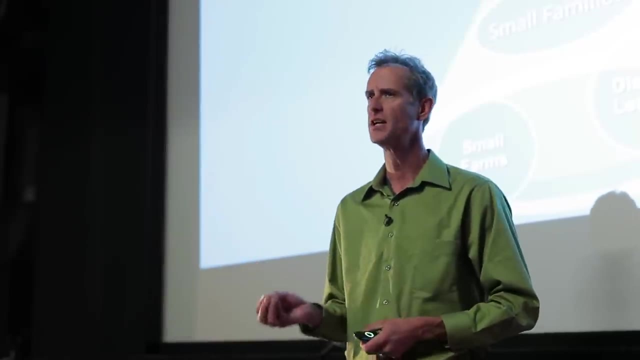 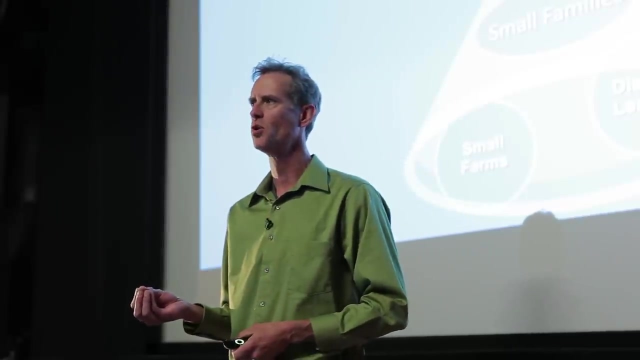 So how effective is this top-down approach? Well, for example, in 2012, the president of Nigeria decreed to his nation that they should only have as many children as they could afford, and he appointed a National Population Commission to determine the feasibility of making birth control a law. 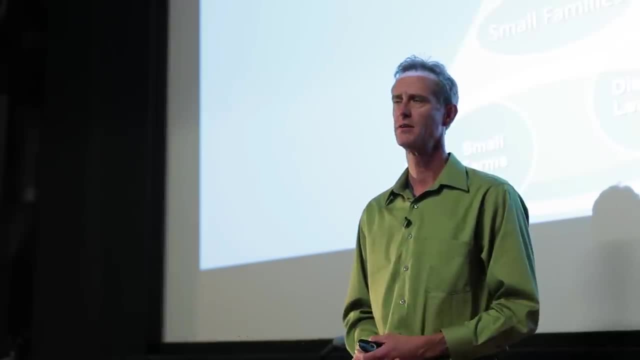 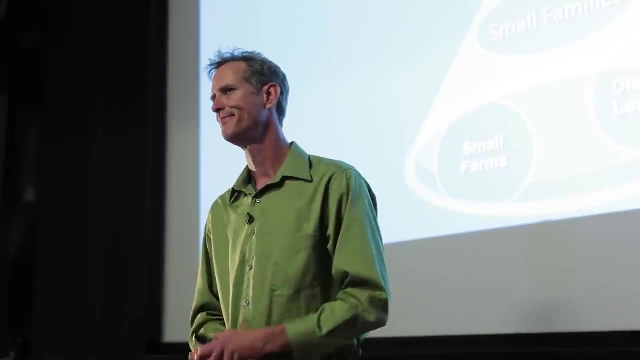 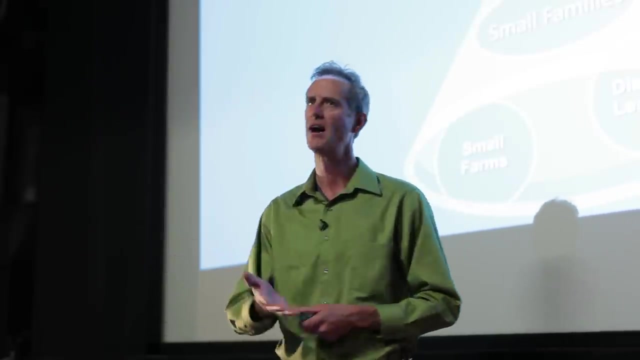 This was met with widespread protests all over the country, for religious reasons, but also a suspicion that the government had the resources but was sequestering them. So what happened here? Well, the government saw a direct connection between families, number of children and 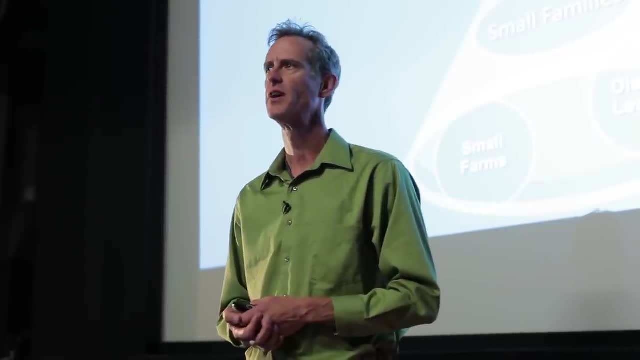 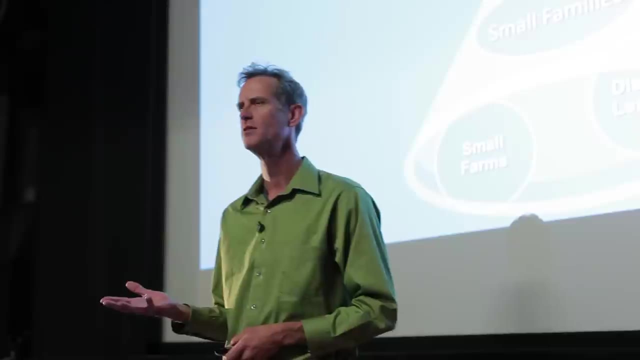 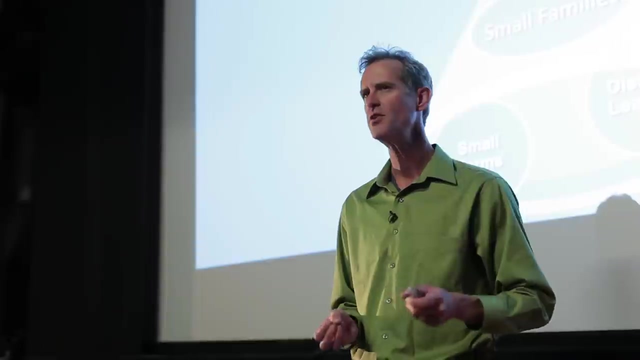 poverty. but the lay public didn't subscribe to this notion and felt that the resources were there but just not available. So a bottom-up approach is needed as well, And in that case the bottom-up approach means that families determine their family size based on individual economics. 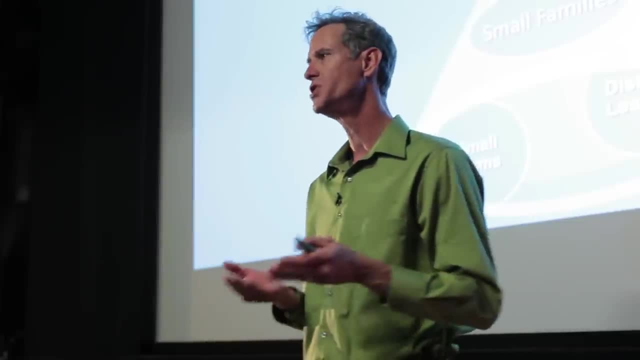 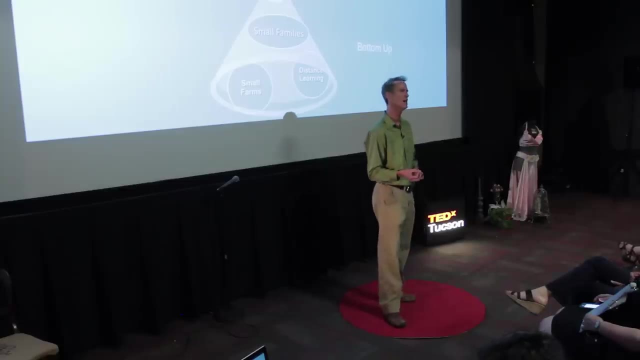 These include access to food, but also education, Okay, And especially for women, because, you see, in developing countries, women who are uneducated tend to be subservient to men and the number of children in a household tends to be determined. 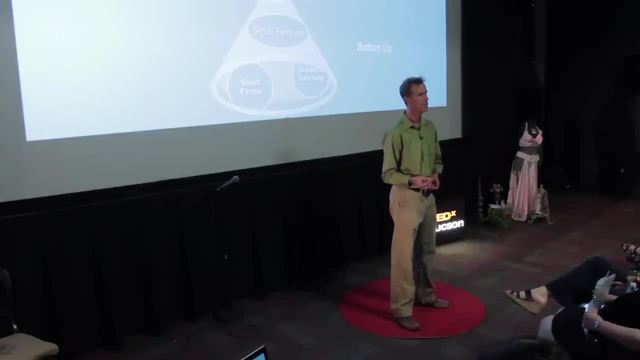 based on what the man wants. Providing education to women in these countries increases their knowledge base but also their confidence, because in a classroom, women have the same obligations and responsibilities as men And upon graduation they can join the workforce. They can increase their personal prosperity, but also national prosperity. 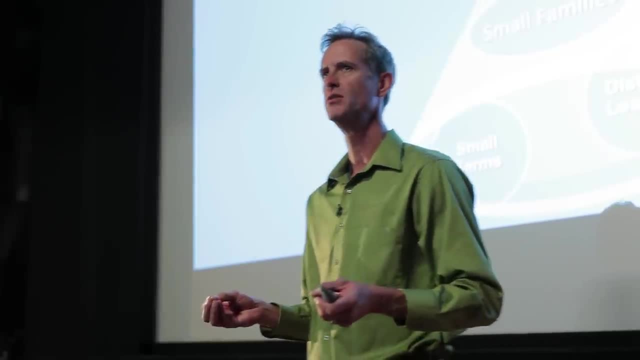 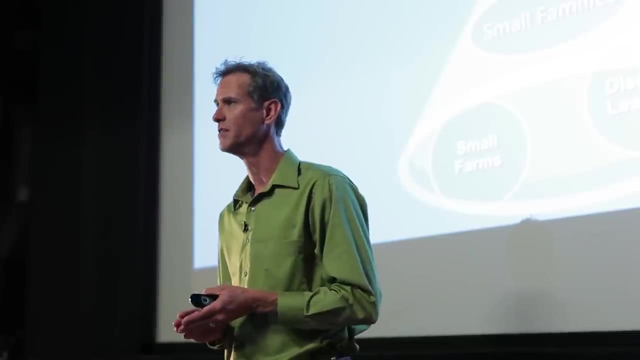 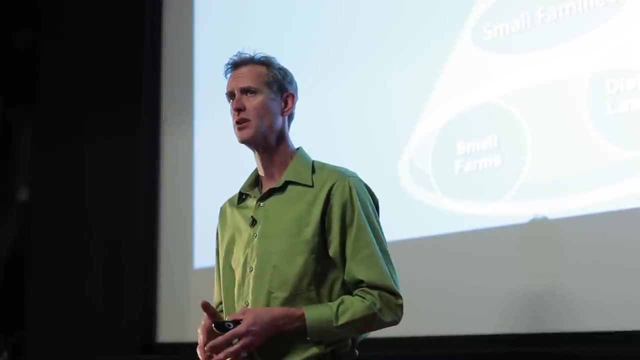 So, with bottlenecks from production to consumption, whether it be for food or education, a decentralized approach would be very effective. In the case of education, that means providing opportunities to learn, Distance learning opportunities, for example, providing computers, Internet access and. 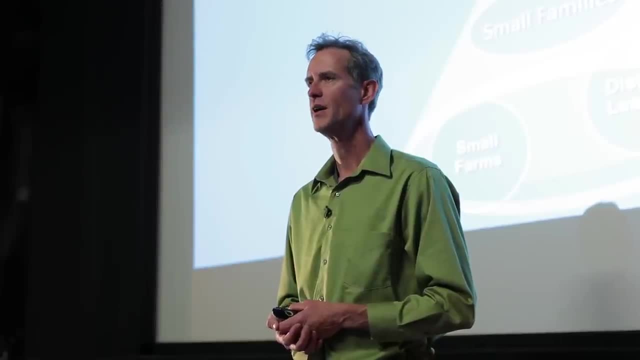 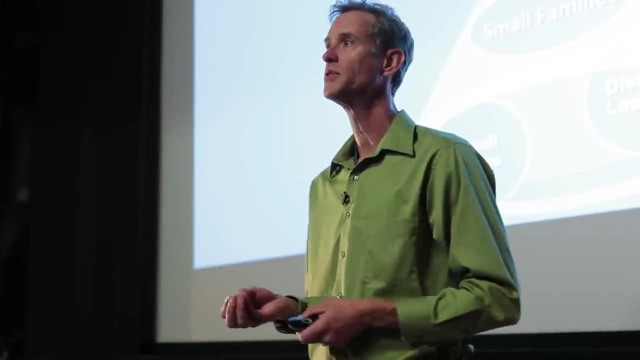 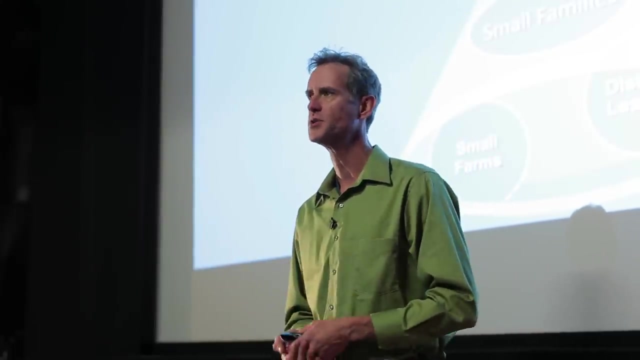 classes that you can take online. And with a third of the food produced all over the planet going wasted, having more and smaller farms would improve access to food, reduce packaging and transport costs and provide jobs, and could also reduce the footprint on the landscape, promoting land. 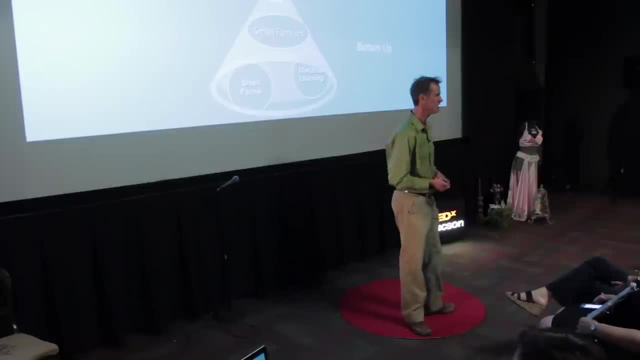 degradation. But you see, a decentralized approach is very effective here, but it's not the only answer, Because in the time of famine, for example, having a centralized resource for food and the ability to distribute that would be vital. Similarly, universal health care would be very important as well, to provide access to. 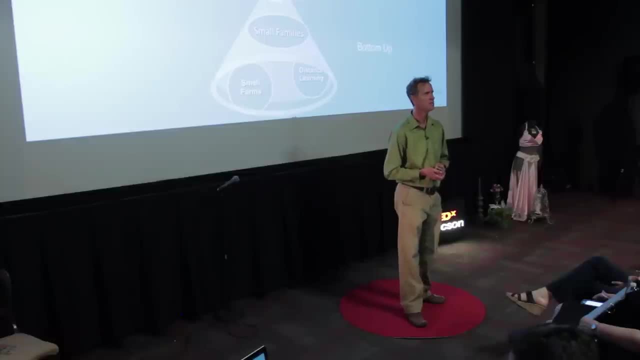 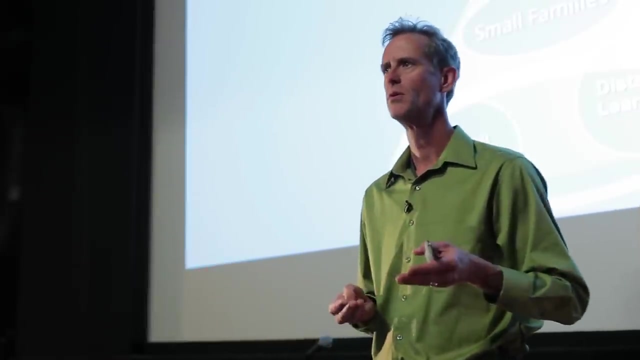 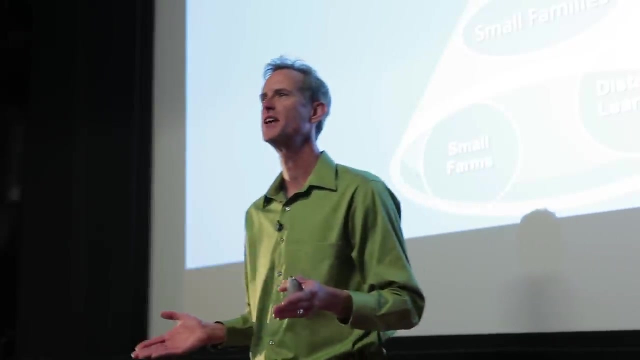 medicines and vaccines to limit the spread of infectious diseases and promote the health of a population. And then, finally, providing education And the incentives to pursue that education Would form a bridge of common purpose between a people and its government. Well, you know, it's easy to take what I've said as abstract concepts. 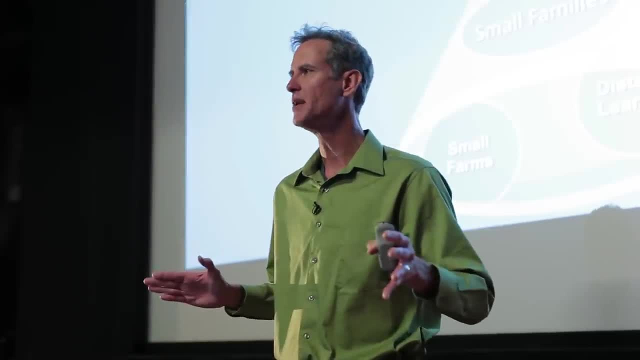 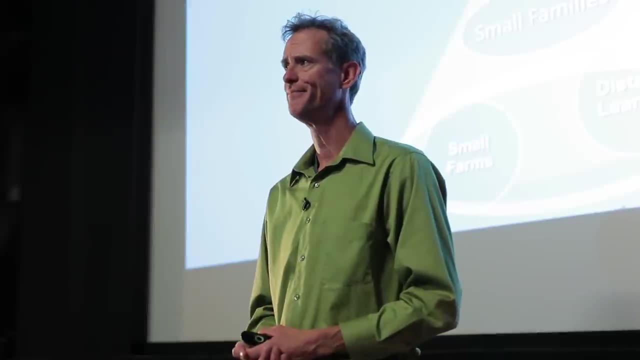 You know, these are things you'd see in a textbook, Something that happens to other people. That is until you go hungry or you have children to feed and you don't have the food to feed them. And let me ask you: what decisions should you make in determining how much food you? 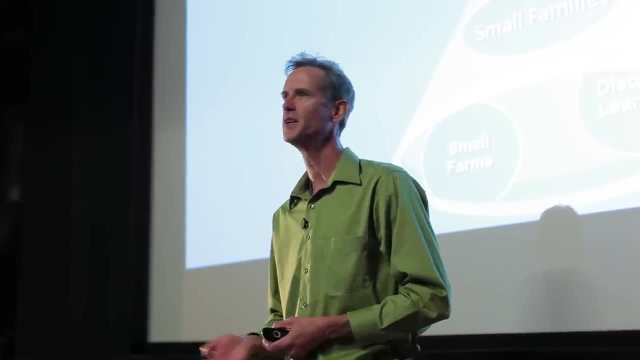 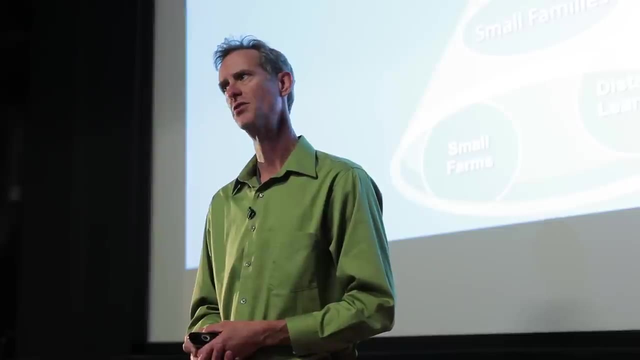 eat how many children you should have? Is it based on what your parents tell you, what your friends tell you, what your religion tells you or what your government tells you? I would suggest consider those things, but also consider the world around you and supply.